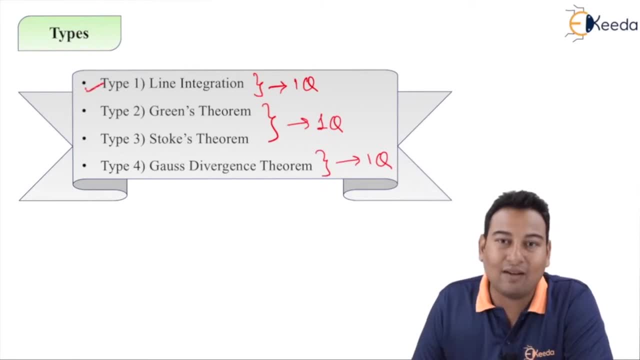 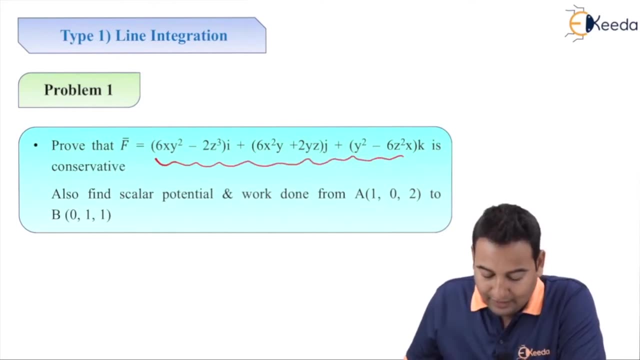 with the first type, that is, line integration. let's have a look on the given problem. proof that f bar is equal to this is f bar given in the problem is conservative. also find scalar potential and work done from a to this in line integration. you can say this is one of the examples that generally comes in the 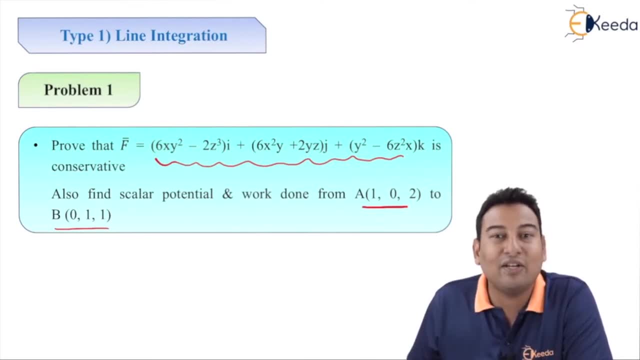 exam out of 10 papers, you can say at least seven to eight papers, you can expect these type of problems. this is very important and generally this comes in the exam for six marks and what i can say: six marks are very sorted here. you can easily get six marks in this question. let's see how. 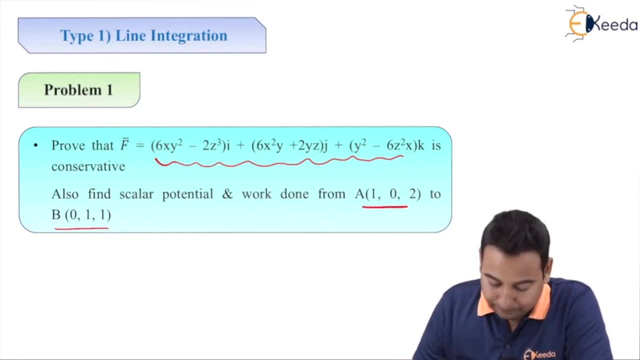 the problem is divided into three parts. let's discuss the parts. the first is we need to proof it is conservative. this is first part. we need to find the scalar potential- that is the second part. and we need to find it out, the work done. that is the third part. for 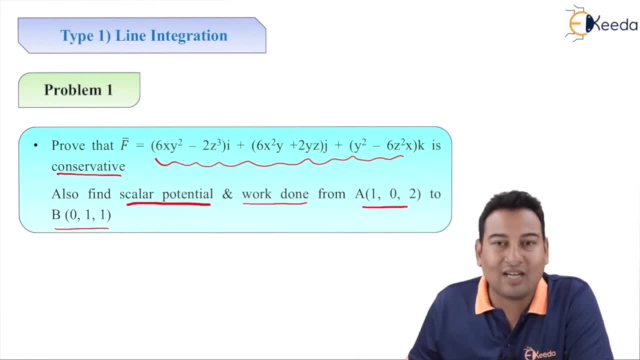 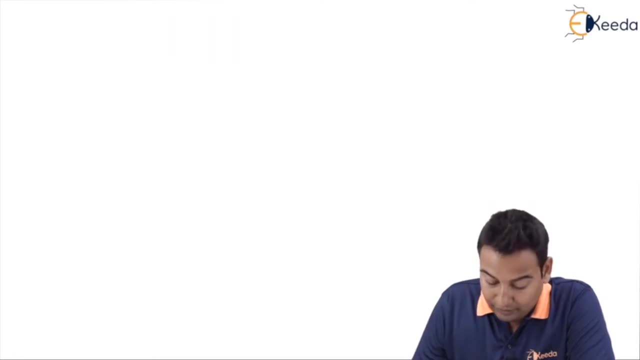 three parts, two marks each, six marks problem. let's start solving the problem. the first part is we need to check whether it is conservative or not. what do you mean by conservative, as discussed in the last videos? conservative or irrotational means? Curl of F bar should be 0. 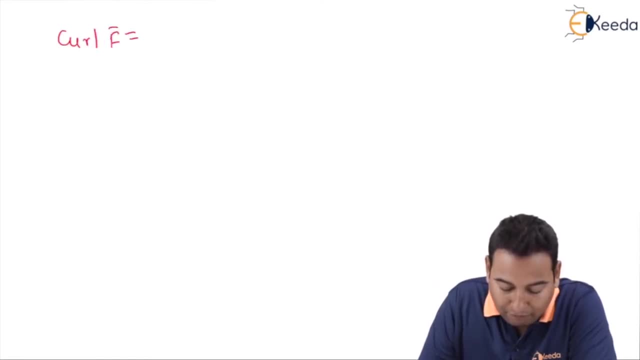 Let's start with the first part. Let me find it out the curl of F bar. If it is 0, I will say the vector is conservative. This is I, This is J, This is K. We do have dou by dou x. 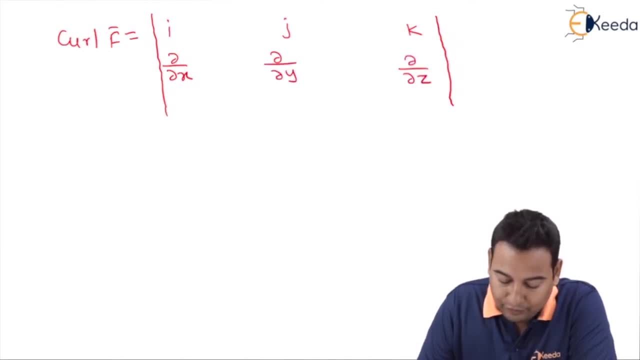 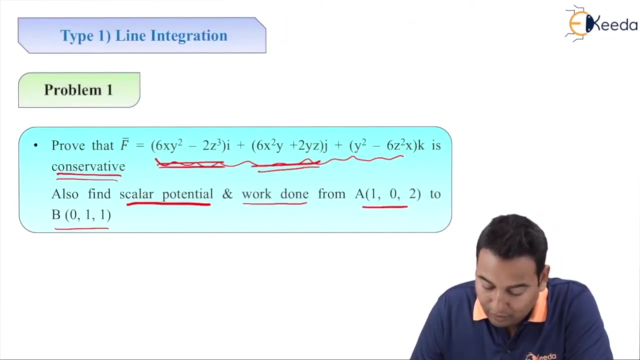 Dou by dou y, Dou by dou z With I. we do have this, That is, 6xy square minus 2z cube. 6xy square minus 2z cube With J. we do have this: 6xy square y plus 2yz. 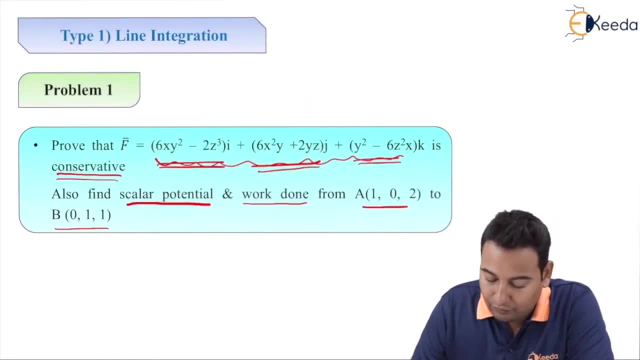 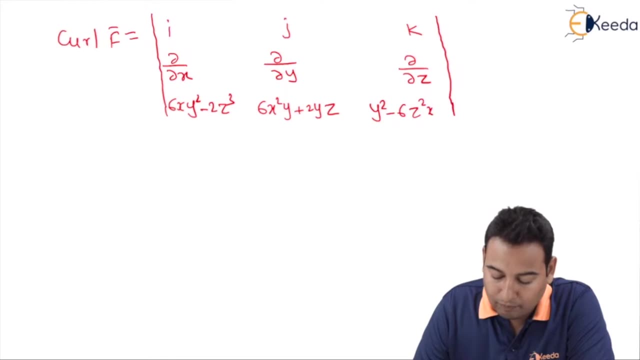 And with K we do have this. That is y square minus 6z square, x. Let me solve this. If the answer is 0, I will conclude: the vectors are conservative. Let's start solving With I Inside. I am going to leave the y column and row. 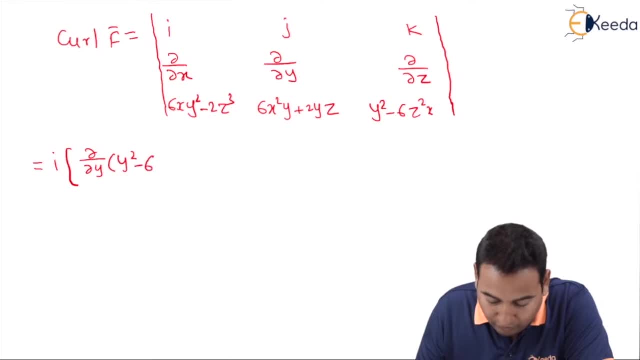 I will get dou by dou y of y square minus 6z square x, First row, this height, And I am going to consider these four terms Minus dou by dou z of 6x square y plus 2yz. Second term in determinant is always minus. 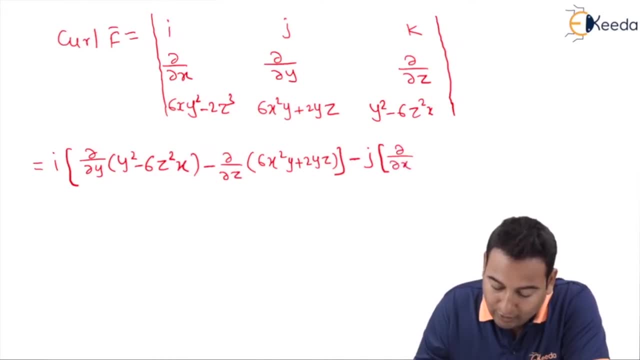 So minus J, I will be getting dou by dou x of y square minus 6z square x, minus dou by dou z of 6xy square minus 2z cube. Finally, plus K, Last term. I am going to leave last column and first row. 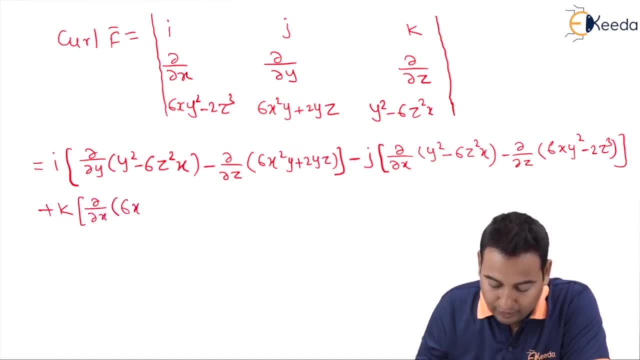 That is dou by dou x of 6xy square y plus 2z cube. And I am going to get dou by dou z of y square minus 6x square y plus 2y z minus dou by dou y of 6xy square minus 2z cube. 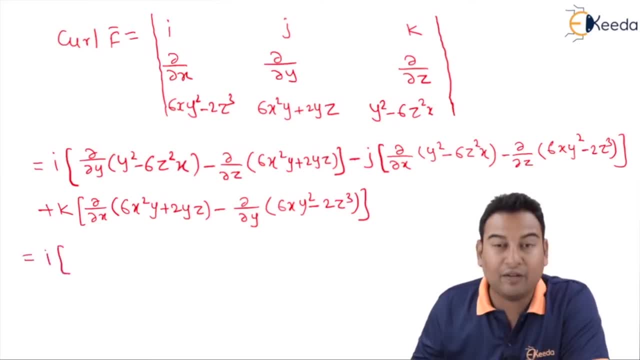 Let's solve this. I Let me differentiate With respect to y. x and z are constant. Here, y square derivative is 2y. This entire term is constant. Therefore its derivative is 0.. Minus With respect to z, its derivative is 0.. 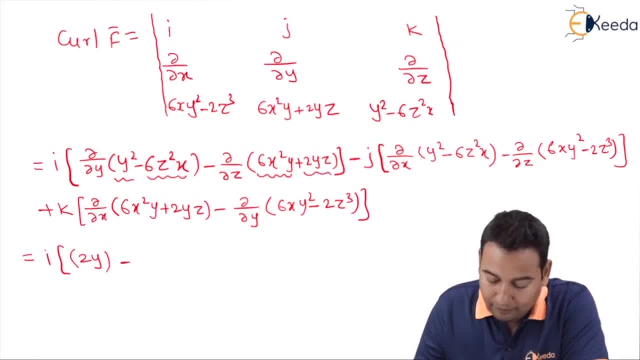 Because with respect to z, x and y, both are constant. Here, with respect to z, 2y is constant, z derivative is 1. Minus j. With respect to x, this is 0. And here, minus 6z, square constant. 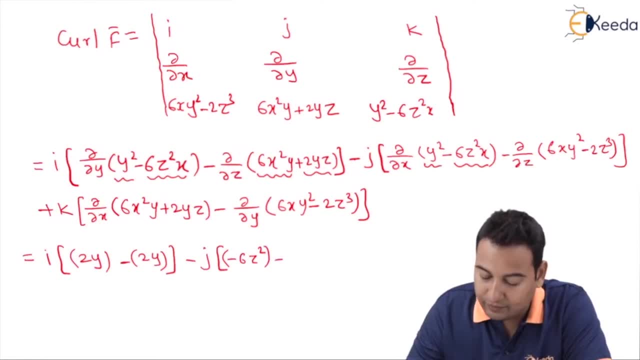 x derivative is 1.. Minus With z, this is 0.. And here it will be minus 2. constant z cube is 3z square, That is, minus 6z square plus k. With respect to x, here 6y is constant. 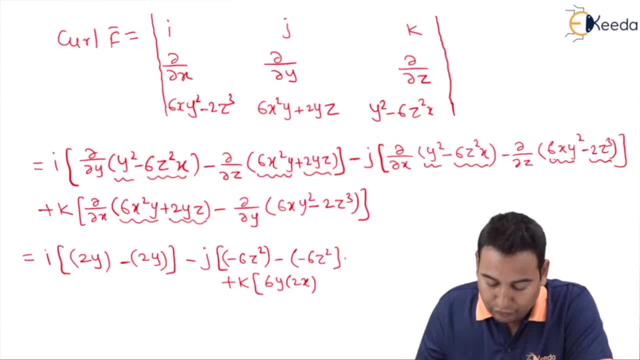 x square derivative is 2x. This derivative is 0.. Minus With respect to y: here 6x is constant. y square is 2x. This derivative is 0.. Let us check. This will be cancelled. 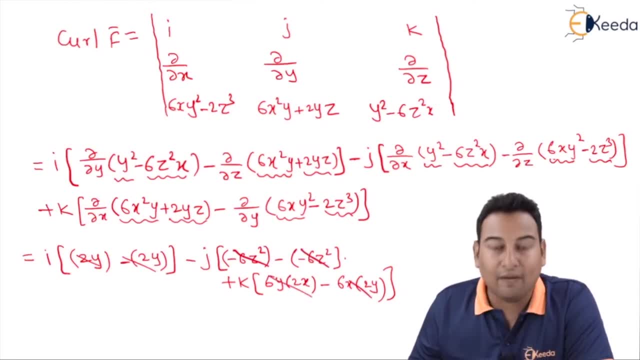 This will be cancelled. This will be cancelled. Everything got cancelled, Which is equal to 0. Since curl of f bar is equal to 0. The vector is conservative, First part is done. Very sorted problem. 2 parts, 2 marks each. 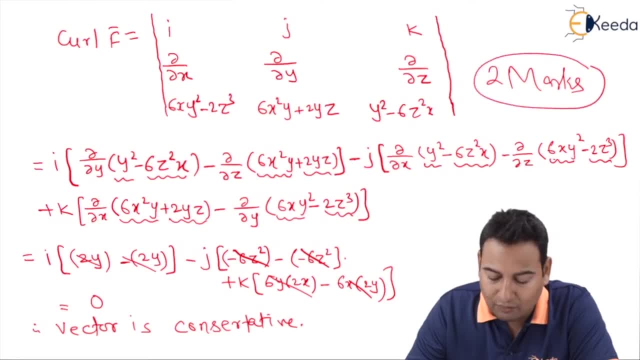 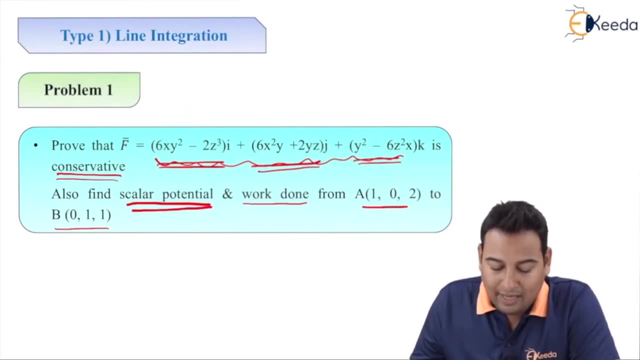 You will score 2 marks for this. 2 marks done, Very sorted problem. Let's discuss the next problem. Let's discuss the next problem, next part: we need to find it out: scalar potential. I'll give you the trick to find scalar potential. 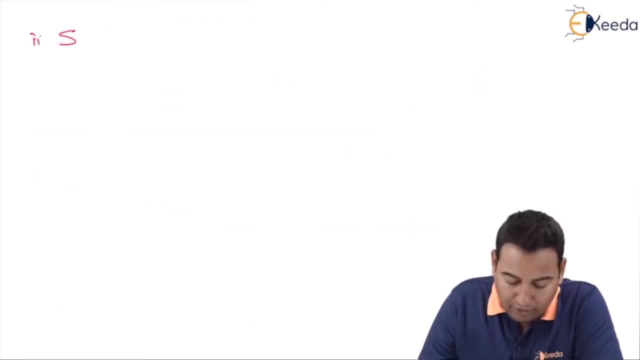 follow that trick and it will be very simple. let's move on number two, scalar potential. that means we need to find it out phi see the trick. first you will write dou phi by dou x. then you're going to write it on dou phi by dou y. 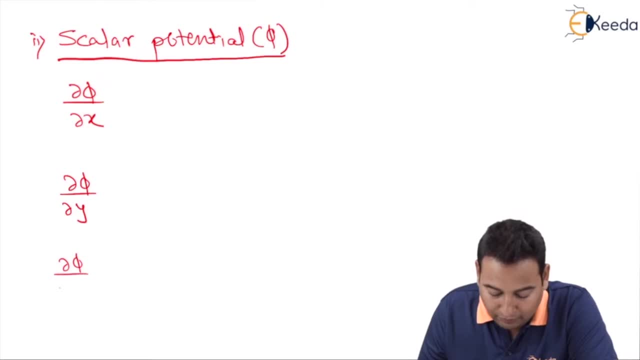 follow the trick and the problem will be simple. finally, write it down. dou phi by dou z. here you're going to write it down: f1, fixed. f1 means whatever with i. that is 6xy square minus 2z cube. this is actually your f1. remember the trick? I'm going to write down f1 here. dou phi by dou y, I'm going to. 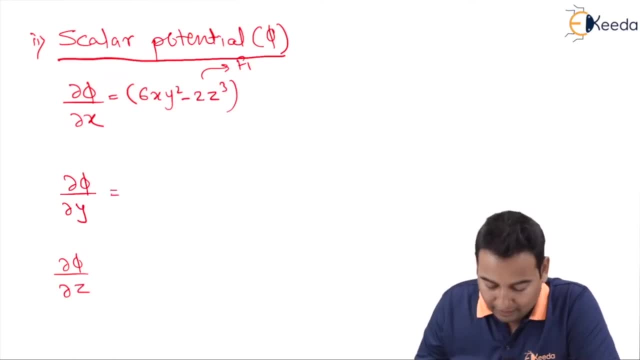 write it down: f2. f2 means whatever with i. f2 means whatever with i. f2 means whatever with i, with the j, which is 6x square y plus 2yz. this is actually your f2. and finally, dou phi by dou z, write it down: f3. f3 means whatever with the k, and that is y square minus 6z square x. 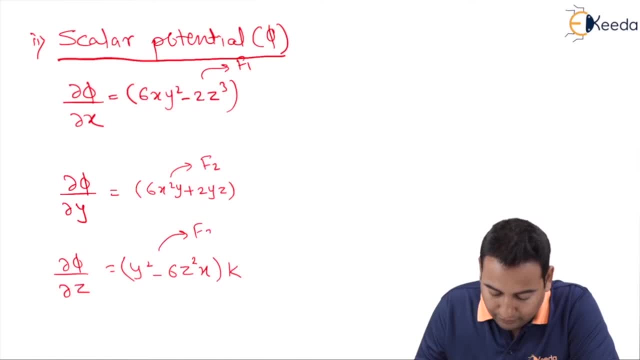 this is your f3- very simple to get phi in three cases. this is your f3- very simple to get phi in three cases. this is your f3: very simple to get phi in three cases. you need to integrate first. here you're going. you need to integrate first. here you're going. 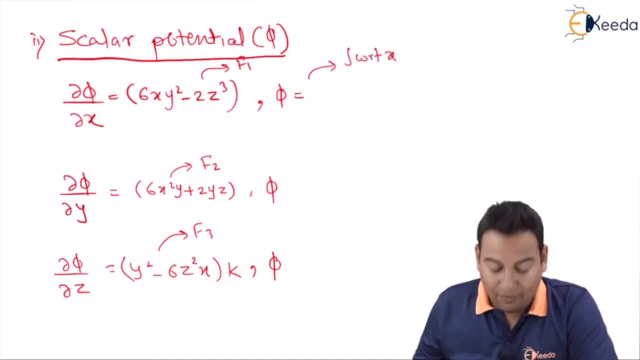 you need to integrate first. here you're going to integrate with respect to x, y with respect to x. to integrate with respect to x, y with respect to x. to integrate with respect to x, y with respect to x, because if you want phi in the denominator, we 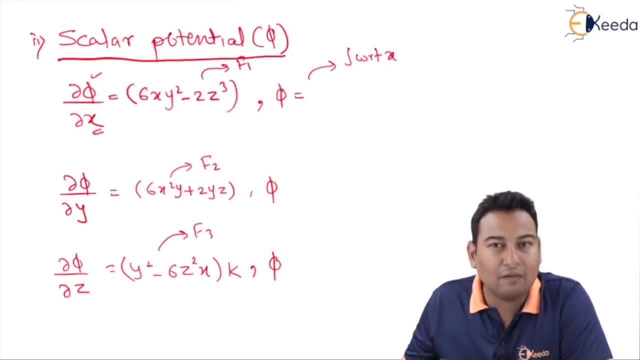 because if you want phi in the denominator we, because if you want phi in the denominator we, do have x. therefore, if you want to phi in the, do have x. therefore, if you want to phi in the, do have x. therefore, if you want to phi in the first case, you need to integrate with respect to x. 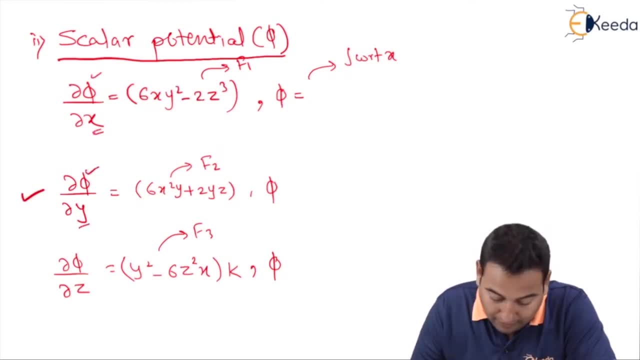 first case you need to integrate with respect to x. first case you need to integrate with respect to x. in the second case, this one, if you want phi. in the second case, this one, if you want phi. in the third case, you need to integrate with respect to Z. let's do that. 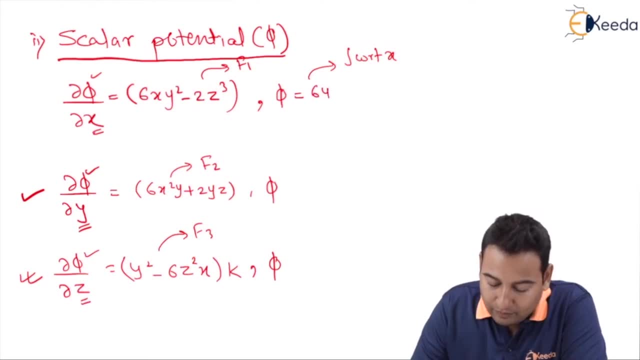 integrate with respect to X. that means 6 Y square constant X. integration is X square by 2 minus 2 Z cube. with respect to X: 2 Z cube is constant. 1 derivative is X, next 5. now I'm going to integrate with respect to Y: 6 X square is constant Y. 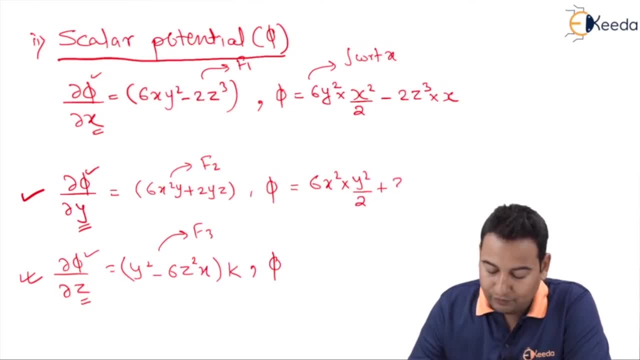 integration is Y square by 2, plus here 2, Z is constant and again Y integration is Y square by 2. for the last part, we're going to integrate this with respect to Y and for the last part, we're going to integrate, with respect to Z, Y square. 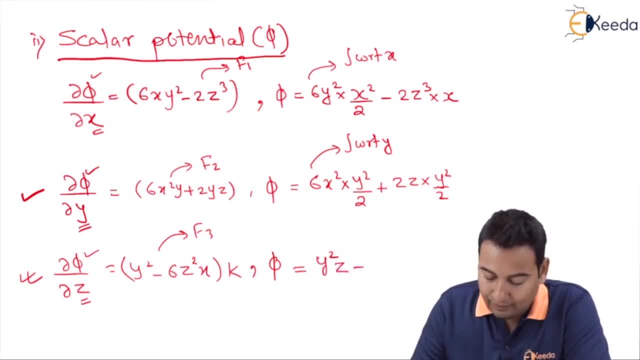 which is constant Y, we are left with one that is Z minus. here, 6 X is constant Z square. integration is Z cube by 3. let's simplify this. this is 3 X square Y square minus 2 X Z cube. this is integration with respect to Z, remember. 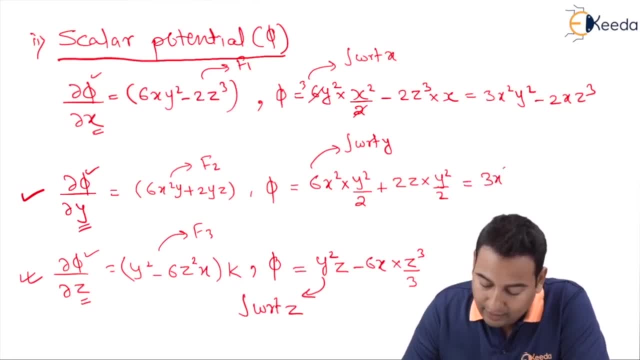 the technique. in the second, again, I'm getting 3 X square, Y square, plus Z Y square. and in the last, I'm getting Y square Z minus 2 X Z, cube friends. so what is total巧? total, hertz of phi, just write all the terms. 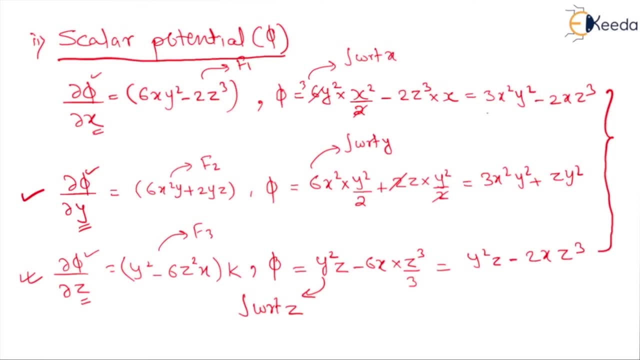 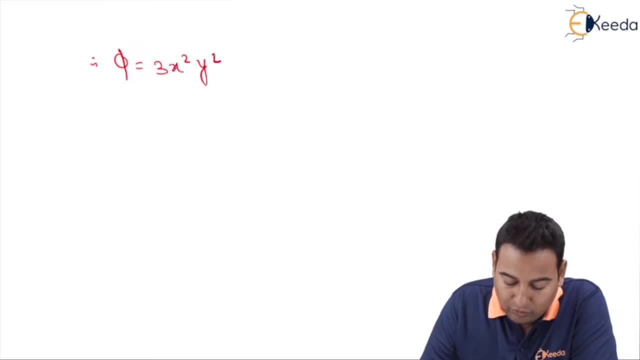 repeated terms will be written once. write all the terms. this is the first term: 10Youb lips parts and 21V Lips. Data values: sum of variance: 3x square y square. therefore, phi is 3x square y square. let's check the next term. 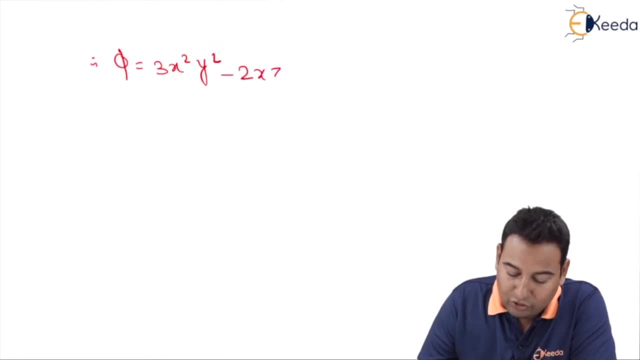 minus 2x z cube. minus 2x z cube. let's move on. 3x square. y square, which we have already covered repeated term, i'm not going to consider. i'm going to consider once only: z y square. we haven't taken, we'll take it now. z y square. let's move on here, friends. y square, z. 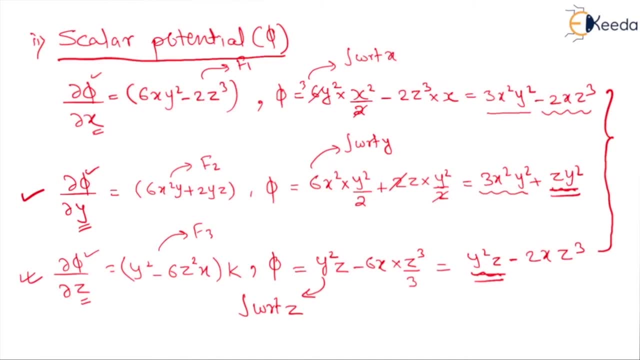 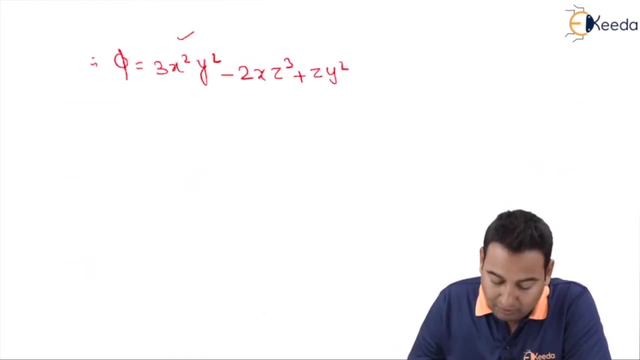 this y square. z is same as z y square. we have already taken. therefore, i'm not going to take the term. and the last term is minus 2x z cube. see this, we have already covered. minus 2x z cube is already covered. therefore, i'm not going to take this. this is my final phi. you will get two marks. 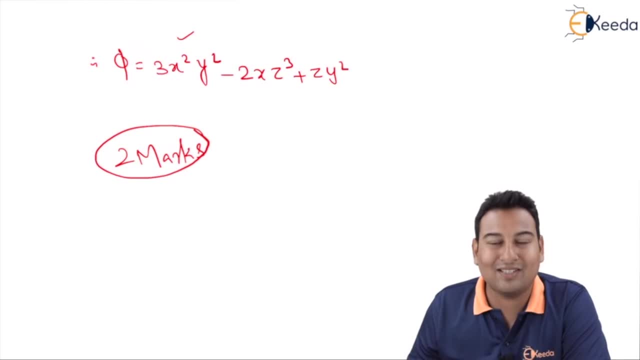 for this. this is your scalar potential. see the technique, remember the technique. the problem will be simple. and the last part is number three. you need to find it out. work done, work done is integration c, f, bar, dot, dr, bar. this is actually your work done. friends, now you might. 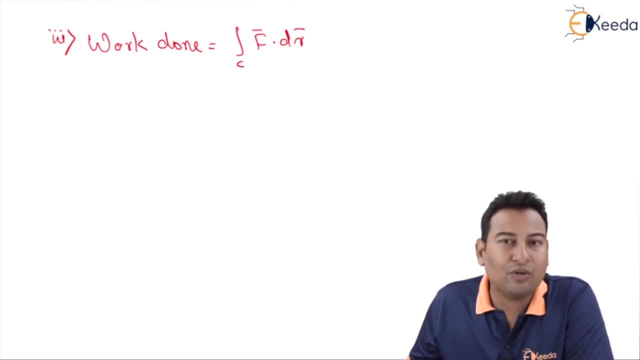 be thinking how to solve this again. i'll give you you a trick to solve this. let's see how to do it. first of all, you're going to to write it down integration. then you're going to write it down derivative. see the pattern i'm writing right on the same way in the example. get full marks, write it down integration. then 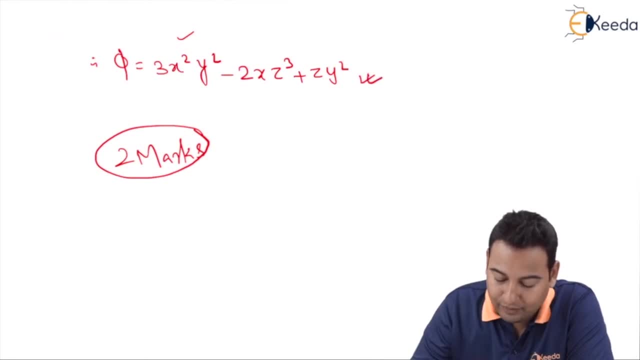 derivative and write it down. the scalar potential that you got. see here this i'm going to write it down: that is 3x square, y square, minus 2x, z cube and plus z y square. same way, please write it down. write down one integration, then derivative, then scalar potential and show this way. 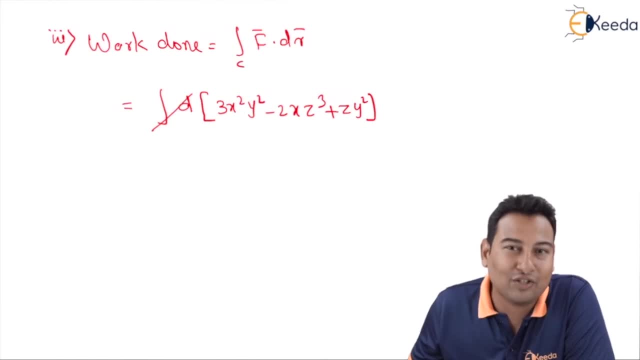 integration and derivative effect will cancel each other. if this got cancelled, you are left with 3x square, y square, 2x z cube plus z y square. what are the limits of the problem? in the problem it is given from 1 comma 0 comma 2 up to 0 comma 1 comma 1. you need to very careful while putting this limit.